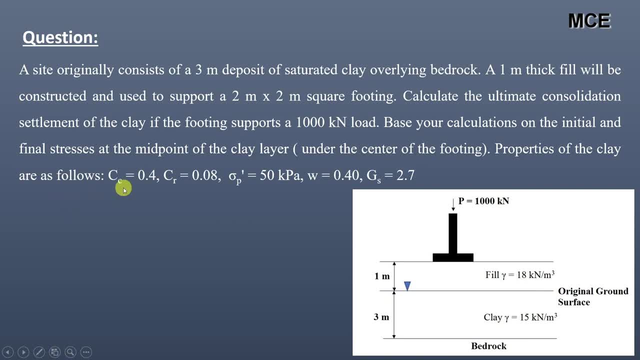 as follows: Compression index is equal to 0.4.. Recompression index is equal to 0.08.. Pre consolidation pressure is equal to 50 kilopascal, Water contact is equal to 0.4 and specific gravity of solid is equal to 2.7.. First we will find the initial effective stress at 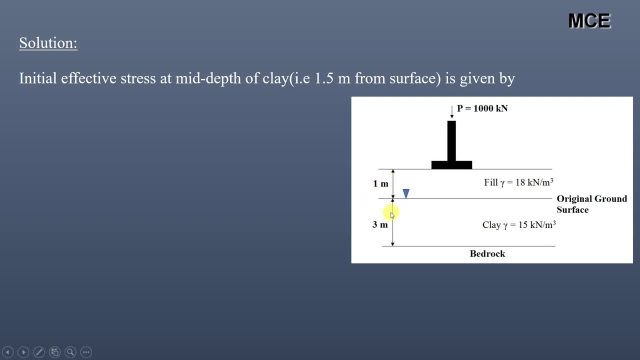 mid depth of clay that is 1.5 meter from the original ground surface and is given by sigma i. prime is equal to gamma saturated minus gamma w, into 1.5, which is equal to 15 minus 9.8. 1, into 1.5, which is equal to 7.8 kilopascal. Stress increase due to fill is given as: 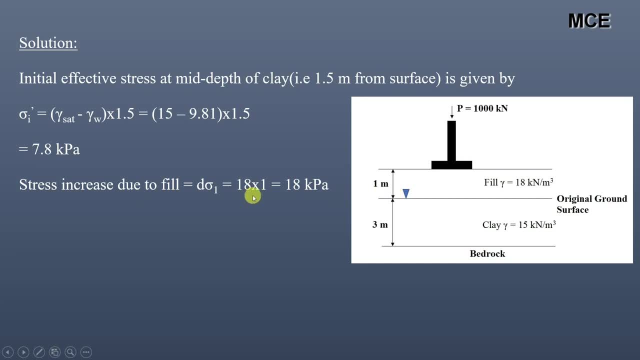 unit weight of fill into depth of fill, which is equal to 18, into 1, which is equal to 18 kilopascal Stress increase at the base of the footing is given as q is equal to p divided by b into l, where p is the load acting on the footing and b and l are the width and length. 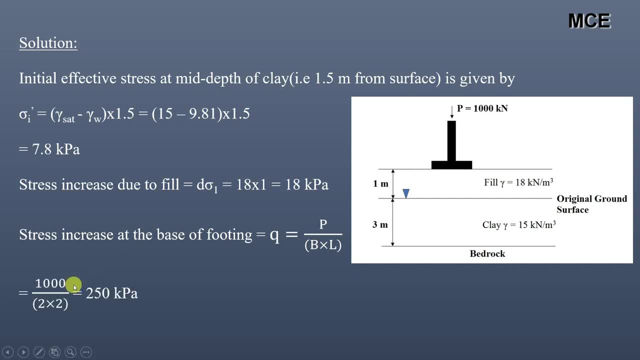 of the footing, Footing values. we get 1000 divided by 2 into 2, which is equal to 50 kilopascal. This is the stress increase at the base of the footing. Since we have to find the stress increase at the mid depth of the clay, exactly under the center of the footing, we will proceed as 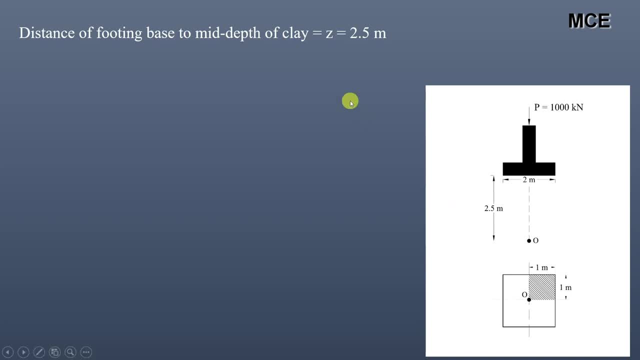 first distance of footing base to the mid depth of clay is equal to. z is equal to 2.5.. Now the footing is divided into four squares of size one meter cross one meter and each of these square shear corners at o. So we will find the stress increase at z is equal to 2.5 meter due to. 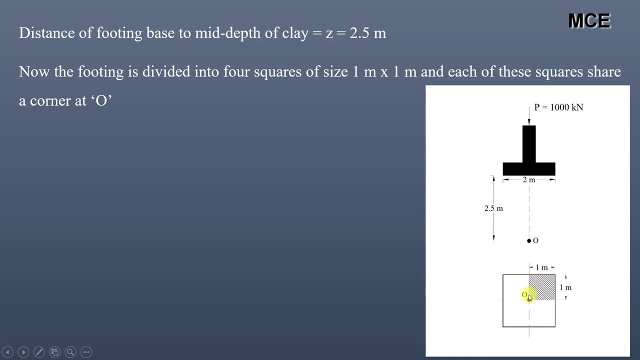 this one meter cross one meter square footing at the corner o. For this one meter cross one meter footing, We have called 1 meter and B is called 1 meter and Z is equal to 2.5 meter. M is equal to A by Z, which. 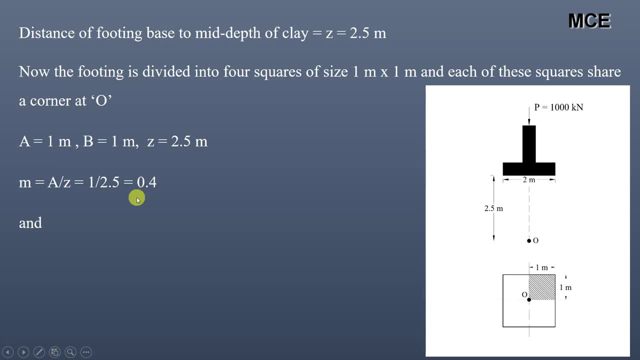 is equal to 1 divided by 2.5, which is equal to 0.4, and N is equal to P divided by Z, which is also equal to 1, divided by 2.5, which is equal to 0.4.. Now we will use the table to find the. 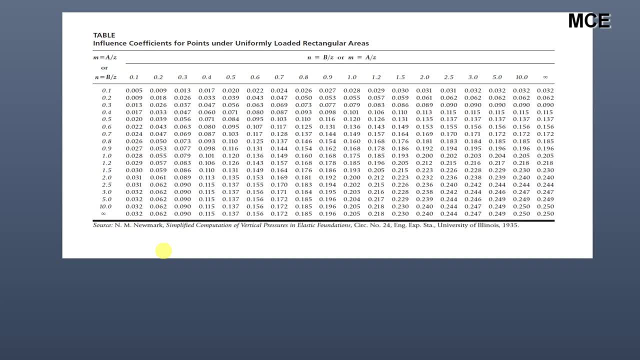 influence coefficient. You can see the figure shows the table for influence coefficients. for points under uniformly loaded rectangular areas, The value of M and N are given in vertical and horizontal rows. So for M is equal to 0.4 and N is equal to 0.4. we can see from the 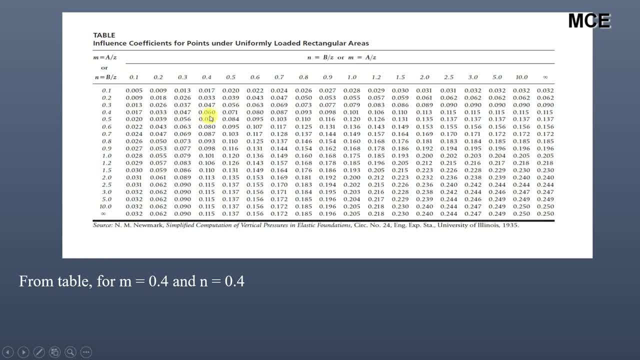 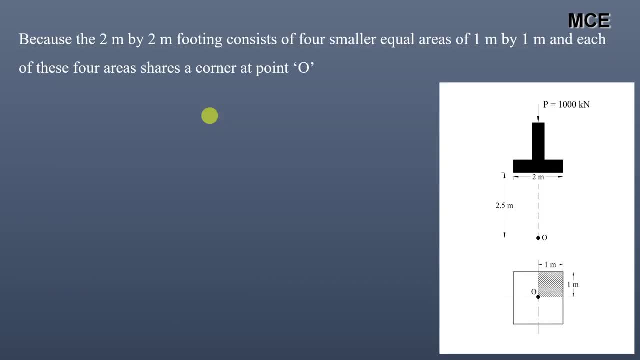 table. the value of I is equal to 0.060.. So influence coefficient is equal to. I is equal to 0.060.. Because our footing consists of four surfaces, we can see that the influence coefficient is equal to I is equal to 0.060.. 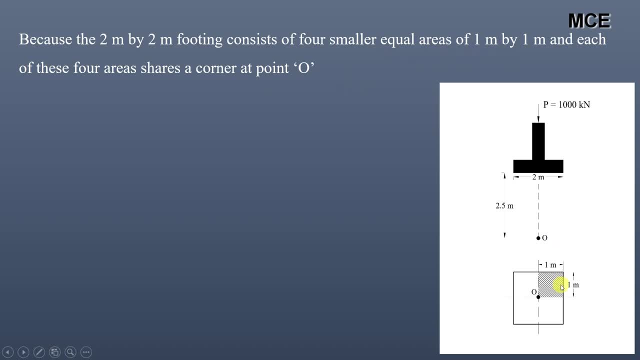 So influence coefficient is equal to I, is equal to 0.060.. Because our footing consists of four smaller equal areas of 1 meter by 1 meter and each of these four areas share a corner at point O. So stress, increase at corner O due to these four areas is equal to 4 into I, into Q, where I is the. 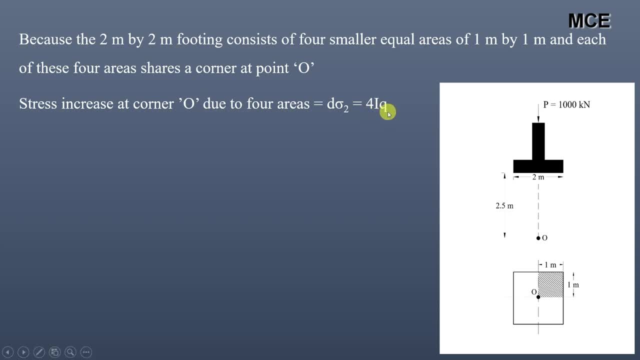 influence coefficient and Q is the stress increase at the base of the footing. So we will get the value equal to 4 into 0.060, into 250, which is equal to 60 kilopascal. So this is the stress increase at the depth of 2.5 meter due to load acting on the footing. 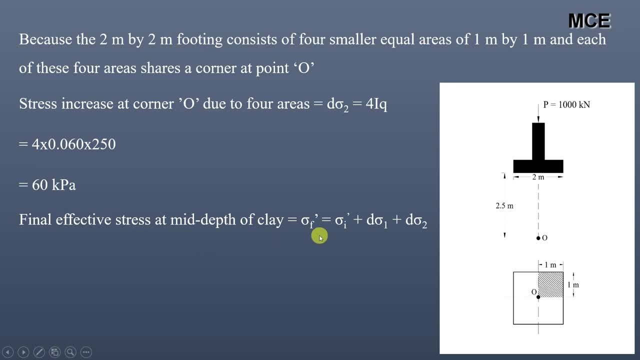 Final effective stress at mid-depth of clay is equal to initial effective stress, plus stress increase due to fill, plus stress increase due to footing, which is equal to 7.8 plus 18 plus 60, which is equal to 85.8 kilopascal. Now, pre-consolidation stress is equal to 85.8 kilopascal. 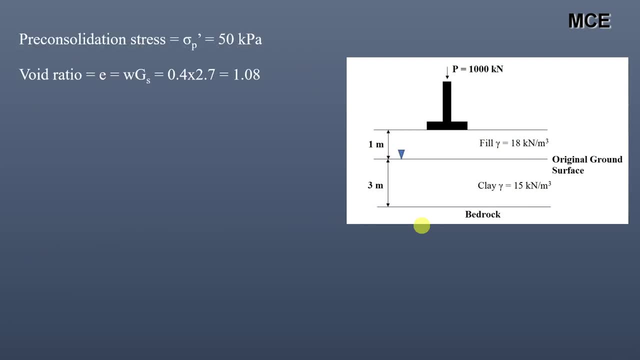 So the stress is given in the question, equal to 50 kilopascal Void ratio, is equal to E, is equal to W into Gs, which is equal to 0.4 times 2.7, which is equal to 1.08.. 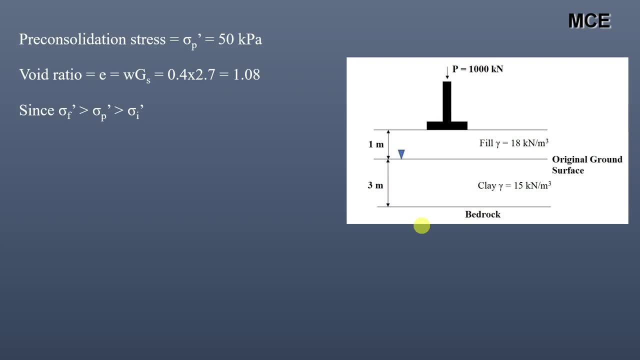 Since final effective stress is greater than pre-consolidation stress, greater than initial effective stress. So consolidation settlement is given: as S is equal to CR into H divided by 1 plus E. log of sigma Prime P divided by sigma prime I plus CC. into H divided by 1 plus E. log of sigma prime F.